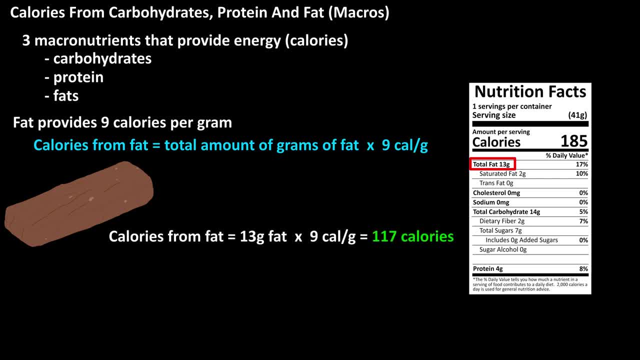 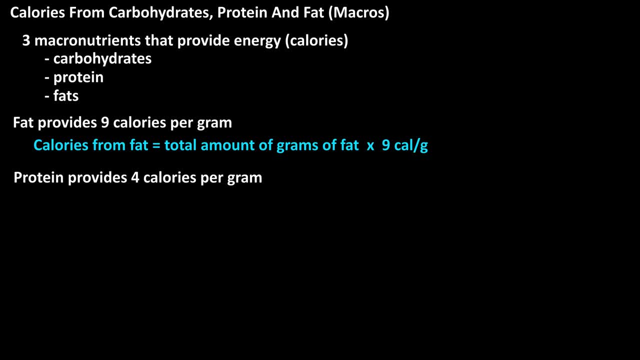 from fat, it would be 13 grams of fat times nine, which equals 117 calories from fat. Now for protein. Protein provides four calories per gram. So to calculate the number of calories from protein for a particular food item, it would be: calories from protein equals the amount of grams. 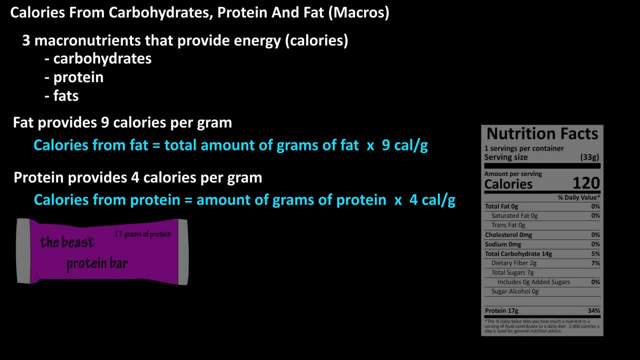 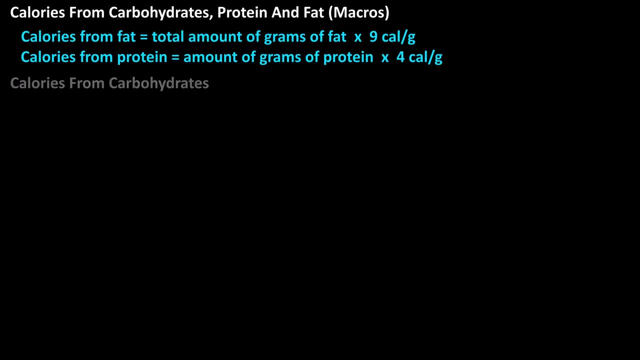 of protein times four. For instance, if you eat a protein bar and on the nutrition label it lists protein at 17 grams, To calculate the number of calories from protein, it would be 17 grams of protein times four, which equals 68 calories from protein. Now for carbohydrates, And this is a little bit more. 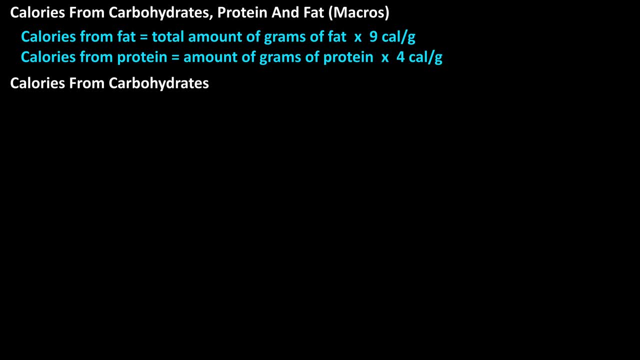 complicated When it comes to calories from carbohydrates. to make things easier, we need to break down carbohydrates into three different types: Regular carbohydrates, fiber and sugar alcohols. Each of these provide different caloric amounts. Here is an example nutrition facts label. 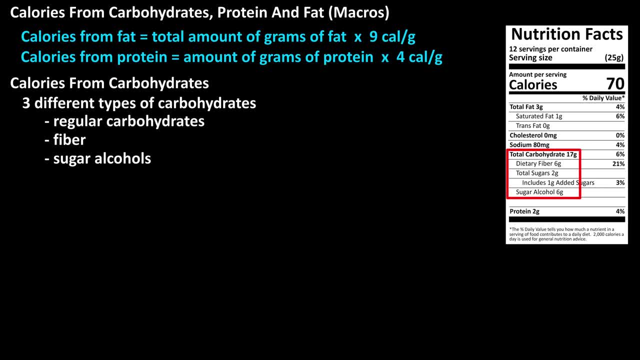 For a one serving size. we see for total carbohydrates it lists 17 grams. This 17 grams of total carbohydrates includes regular carbohydrates, fiber and sugar alcohols. To find the number of regular carbohydrates we need to deduct the six grams of fiber and the six grams of sugar alcohols that the label lists Regular. 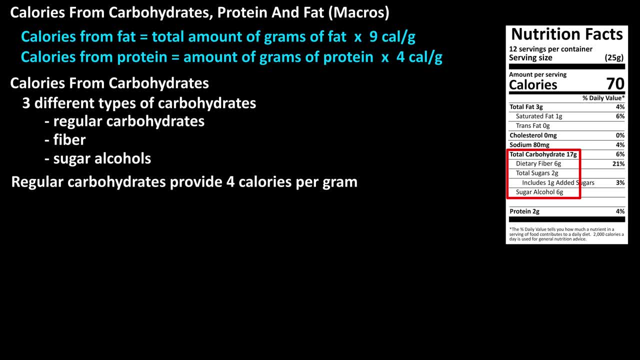 carbohydrates provide four calories per gram. So the formula to calculate the number of calories from regular carbohydrates is: calories from regular carbohydrates equals the quantity total grams of carbohydrates Minus the grams of fiber, minus the grams of sugar, alcohols, times four From our example nutrition. 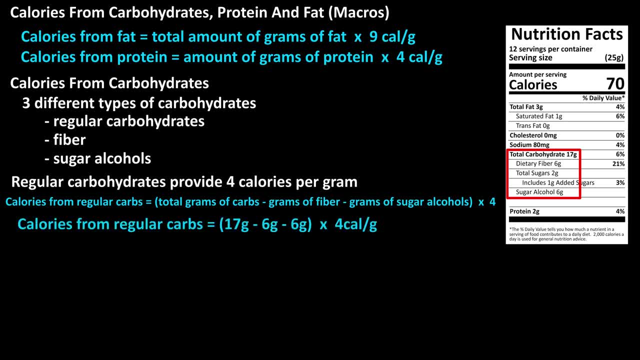 label. we have 17 grams minus six grams, minus six grams, which equals five grams. So five grams of regular carbohydrates. Five grams of regular carbohydrates times four calories per gram equals 20 calories. So we have 20 calories from regular carbohydrates. Now for fiber. Fiber is a 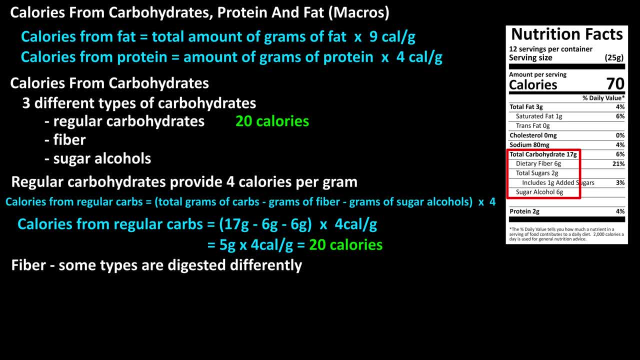 type of carbohydrate that is not digestible in the way other carbohydrates are digestible, And there are two types of fiber: Soluble fiber and insoluble fiber. Insoluble fiber does not provide any calories. However, soluble fiber is broken down by bacteria in the large intestine and does provide 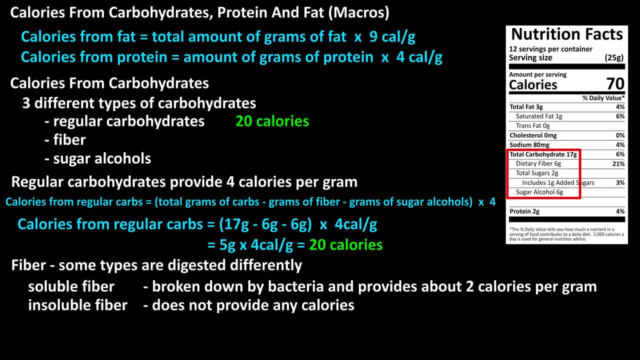 some calories. Soluble fiber provides about two calories per gram. In most cases, on nutrition labels the total amount of fiber is listed, Not the amount of soluble and insoluble fiber. So it's usually a good idea to just assign a few calories per gram of fiber to be safe. On our example, probably one can simply just Speck this into分よろ: cosmic singers. 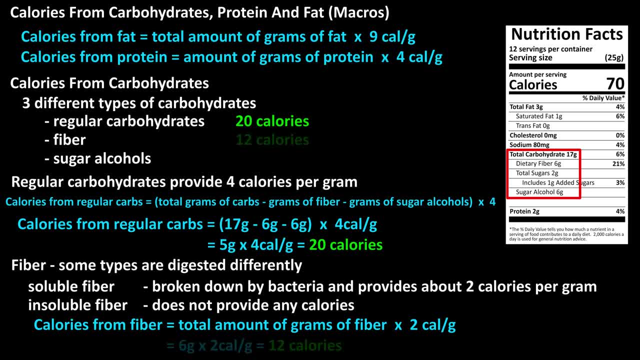 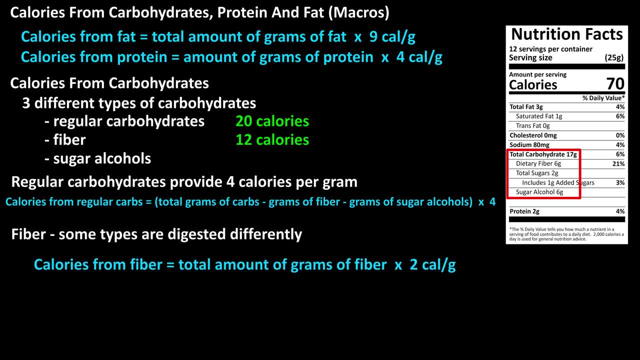 On our example label. it lists the fiber at 6 grams. so we just multiply that: 6 grams times 2 calories per gram, which equals 12 calories from fiber. Now for sugar alcohols. Sugar alcohols are a type of carbohydrate that contains 0 to 3 calories per gram, depending. 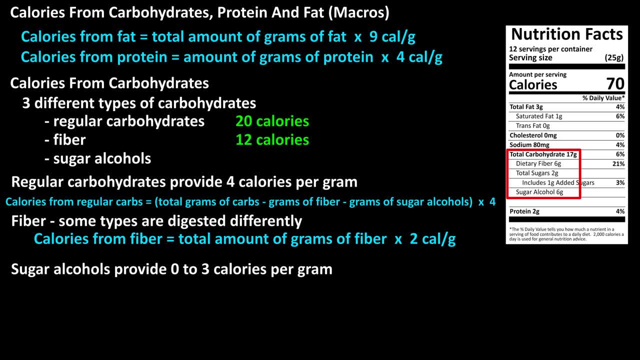 on the type of sugar alcohol. To make it easier to calculate, just estimate 2 calories per gram for sugar alcohols. On our example label it lists the sugar alcohols at 6 grams, so we just multiply that 6 grams. 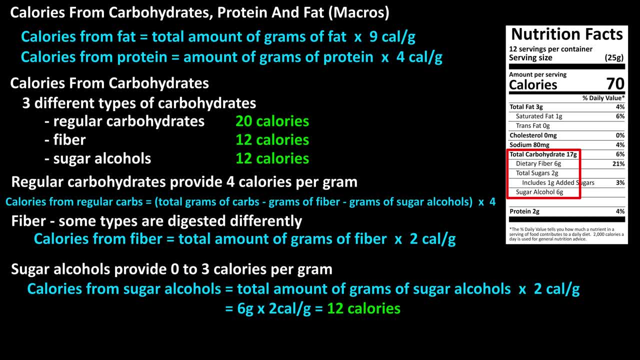 times 2 calories per gram, which equals 12 calories from sugar alcohols. And one note: sugar alcohols are not required to be listed on food labels unless a statement is made on the packaging label about the health effects of sugar alcohols or sugar. 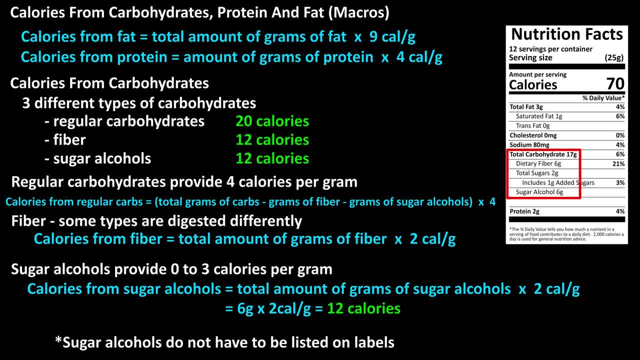 If there's no listing for sugar alcohols, then just ignore calculating. Now we can add up the total calories from all the carbohydrates. We have 20 calories from regular carbohydrates, plus 12 calories from fiber, plus 12 calories from sugar alcohols. 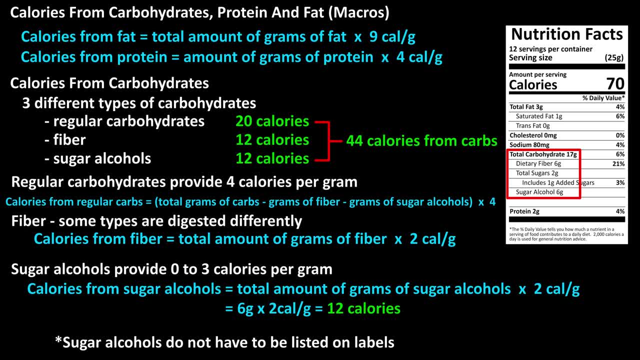 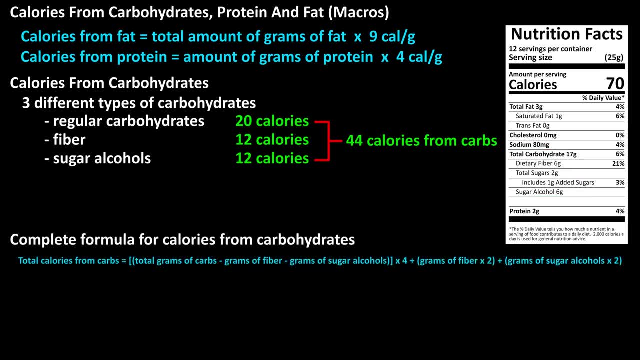 Which gives us a total of 410.. 44 total calories from carbohydrates. The complete formula for total calories from carbohydrates is: total calories from carbohydrates equals the quantity total grams of carbohydrates minus the grams of fiber, minus the grams of sugar. alcohols: times 4, plus the grams of fiber, times 2, plus the grams of sugar. 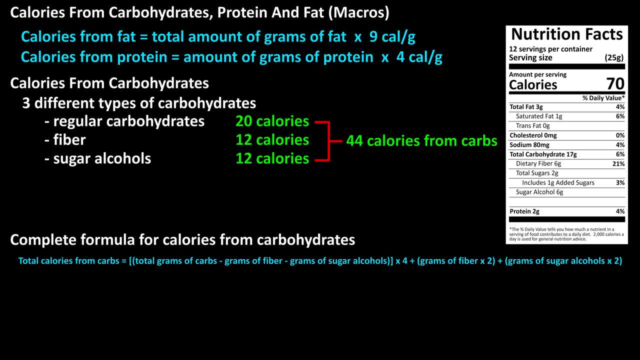 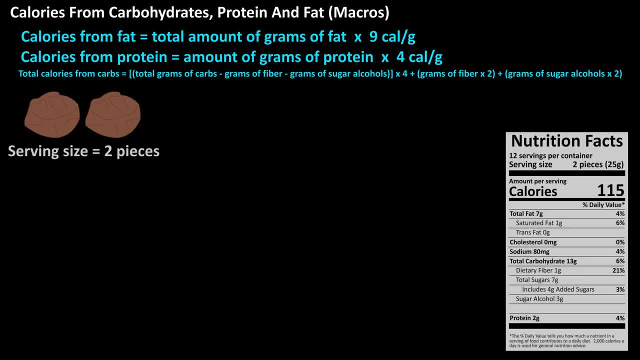 alcohols times 2.. One thing to keep in mind is the data listed on the nutrition label is always for a serving size. If, for example, you're going to eat some chocolate candies, I've listed the serving size at 2 pieces, at 25 grams, with 7 grams of fat: 2 grams. 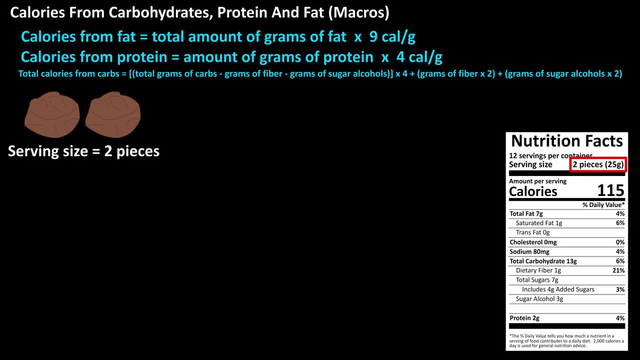 of protein and 13 grams of carbohydrates, with 1 gram of fiber and 3 grams of sugar alcohols. for that serving size I've done the calculation for the total calories and the breakdown of calories from the macronutrients. 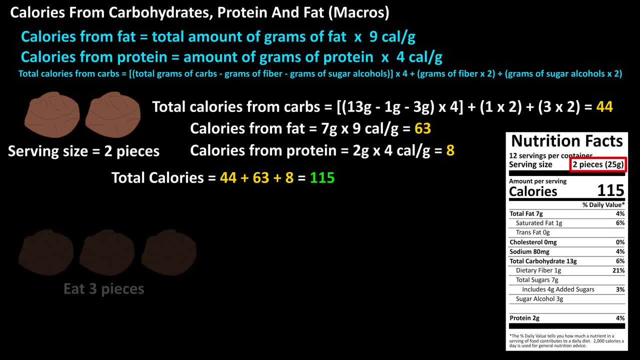 which equals 115 total calories. If you ate 3 pieces, you would have to adjust for that. To do that, you would divide the number of pieces you ate by the serving size: 3 pieces divided by 2 pieces, which is 1.5..